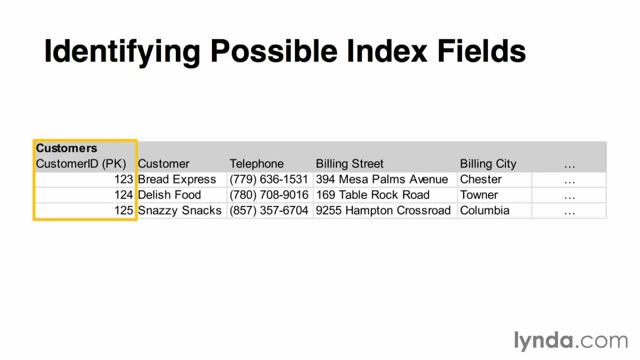 This makes it easy to pull up listings of invoices associated with that customer, since all the invoices will reference the customer ID value. But what happens if the customer calls requesting a status update on a recently placed order, Since it's unlikely that they'll know their ID number? 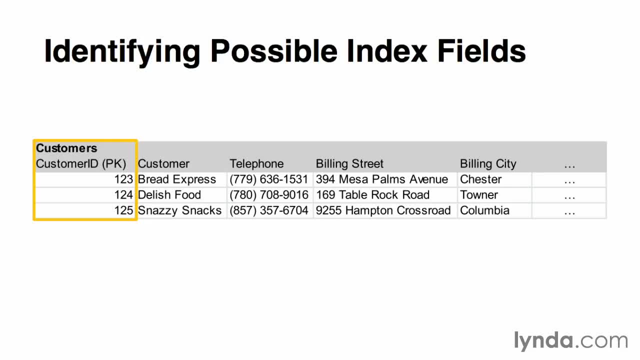 the service representative will need an alternate way of quickly finding their order. We could find all of the orders placed by people with the same last name, or maybe our business procedure indicates that the customer provides us with their telephone number, or maybe the last four digits of the credit card they used. 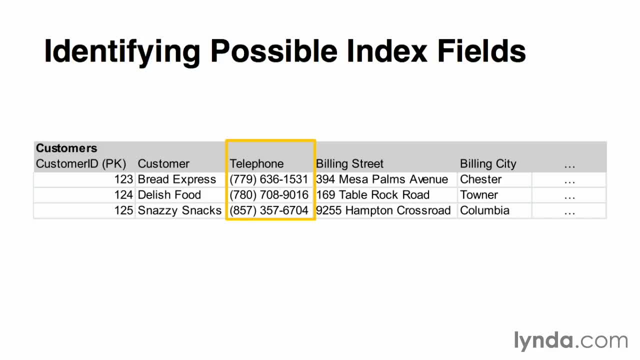 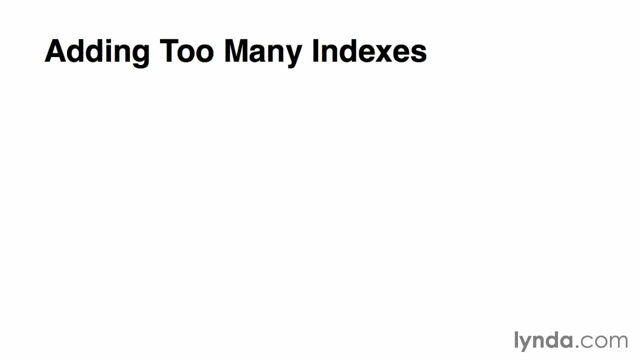 Each of these values could be used to search the database to find their order information, and all our candidates for possible feedbacks would have to use these same fields to add indexes on. The obvious question now becomes: why don't we add indexes to all of our columns? 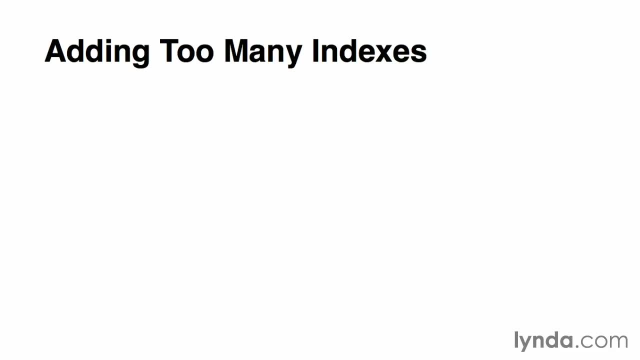 The reason we want to be selective in which columns we decide to add indexes on is because indexes will slow down the database's ability to add new records. If you think about adding indexes as printing additional telephone directories sorted by different values, then you can quickly see that adding a new person to the phone book. 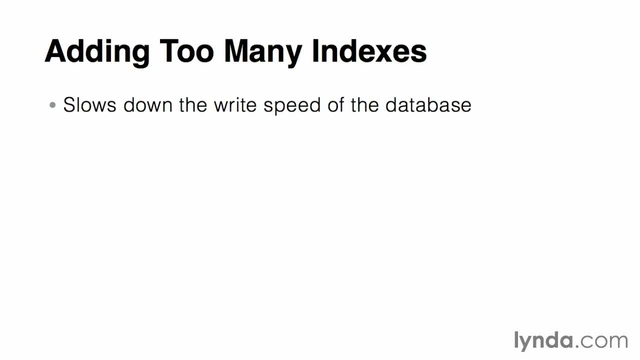 really means that you need to update all of the index directories as well. This is the same in the database, So every time you add a new record to a table, or update or delete an existing record, all of the indexes need to be rebuilt. 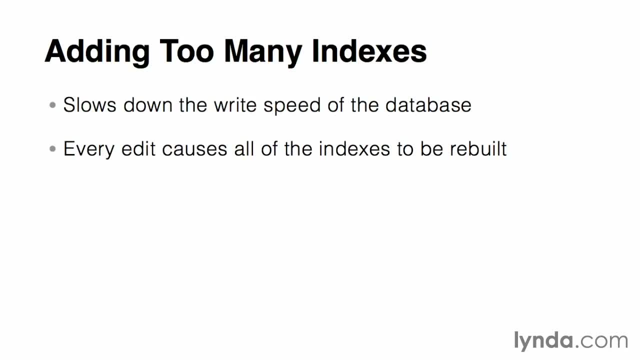 If you have too many indexes, this can dramatically impact the speed at which the database can add new records to a table. It's important to note that not having an index on a column doesn't prevent you from searching the database by that field, Just like searching through the phone book armed with only a telephone number. 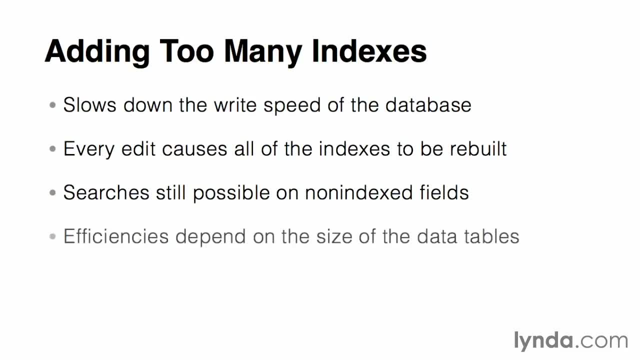 the process is still doable. it's just not very efficient. Depending on the size of your data tables and the types of questions you typically ask of the data, adding indexes might not offer any noticeable speed increases. So that's how indexes work in a relational database. 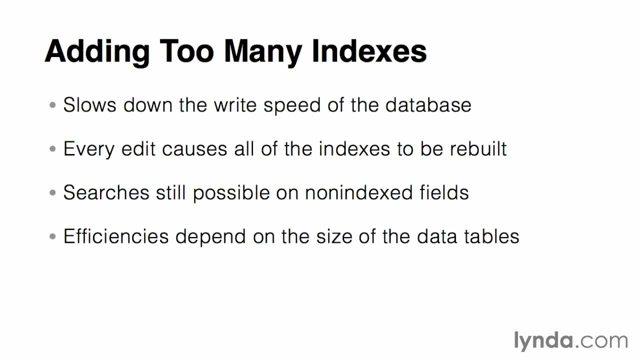 They help the system find specific pieces of information quickly, but they do so at the speed at which a new record can get added to the database. As a final update to our table design worksheets, go through and identify all of the fields within your tables.